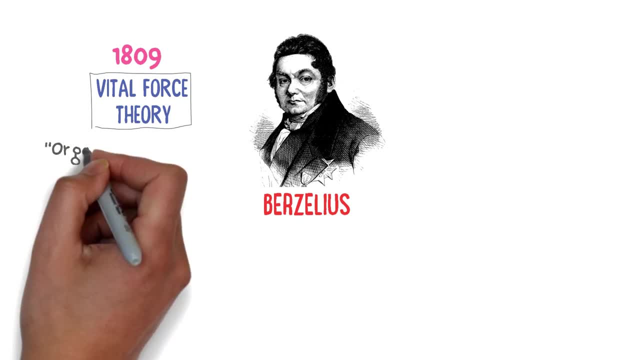 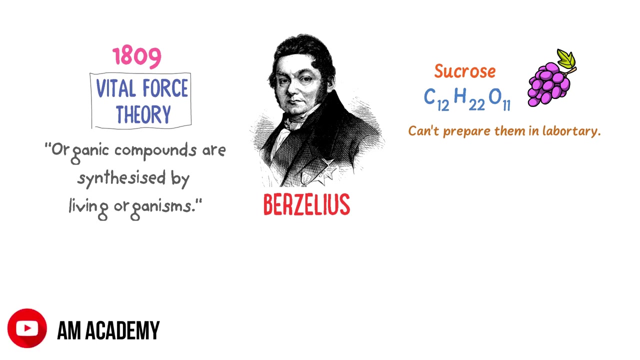 in 1809.. This theory states that organic compounds are synthesized by living organisms and it cannot be prepared. For example, according to this theory, carbohydrates like sucrose C12H22O11 is only synthesized by plants. We cannot prepare them in the laboratory. Secondly, 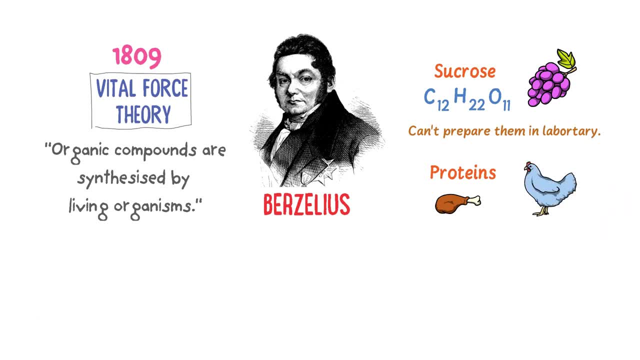 proteins are only synthesized by animals. Also, we cannot prepare them in the laboratory. They believed that God-given power is present only in living organisms, which is responsible for the synthesis of organic compounds. Due to this belief, the vast field of organic compounds was not discovered. 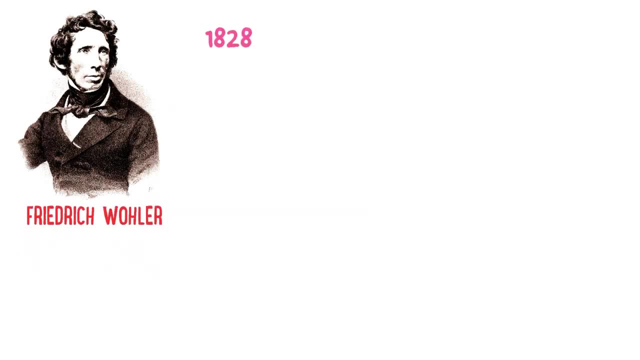 But a German scientist, Friedrich Uhler, in 1828 broke the Vital Force Theory. He prepared the first organic compound, urea, in a laboratory. He took ammonium cyanide and after heating it converted to urea. Urea is an organic compound. 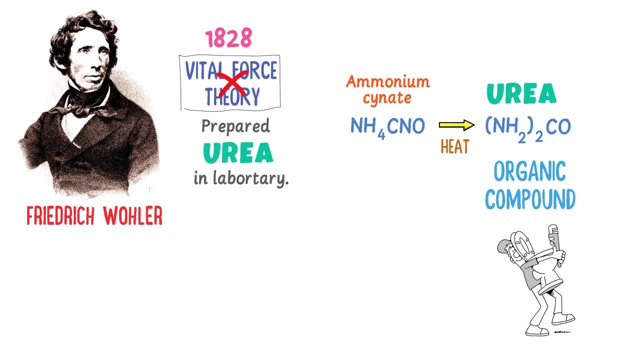 which is found and waste products of living organisms like human beings. He noted down that this is the first chemical reaction of organic compounds. Secondly, urea is the first man-made organic compound. Due to this important milestone, Friedrich Uhler is called as the father of organic chemistry. Thus he opened a new chapter in the chemistry. 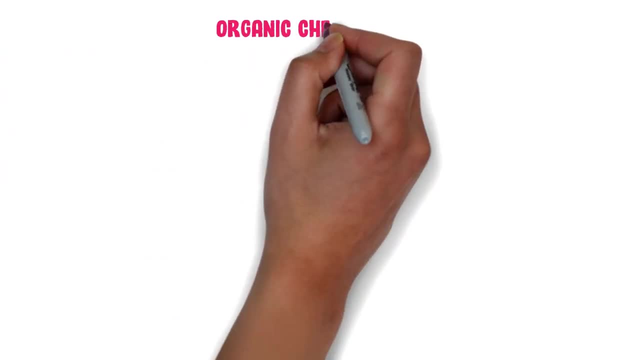 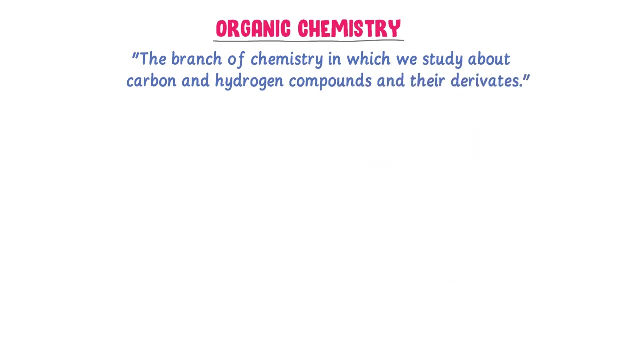 called organic chemistry. Now, what is organic chemistry? The branch of chemistry in which we study about carbon and hydrogen compounds and their derivatives is called organic chemistry. For example, we study about two areas in organic chemistry. Firstly, we study about carbon and hydrogen compounds. Next, we study about theсеal components, For example, we study about carbon and 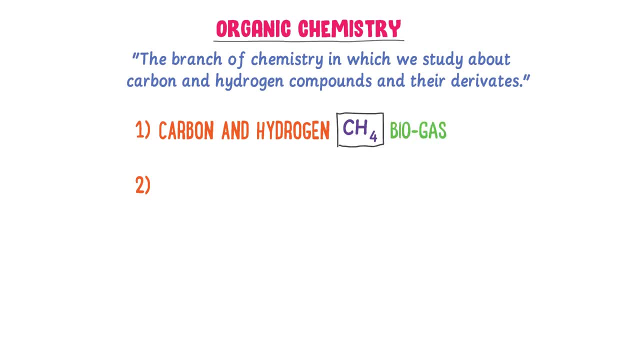 like CH4, which is commonly known as a biogas. Secondly, we study about carbon and hydrogen derivatives, For instance, consider CH4 or methane. It is organic compound and we can convert it into carbon tetrabromide, CBR4.